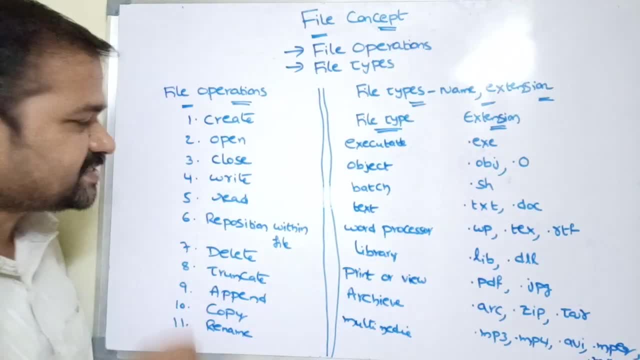 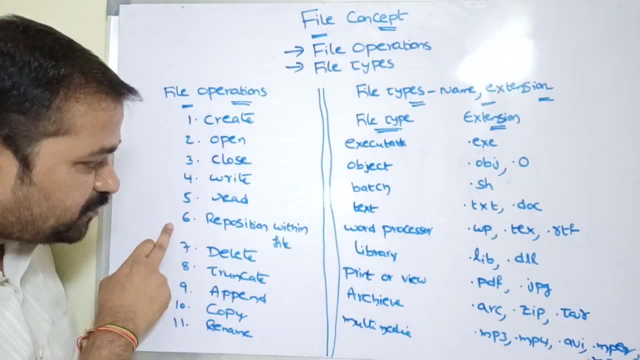 Totally we have 11 operations, 11 important operations. First one is create. second one is open. third one close. fourth one write. fifth one read. sixth one reposition within a file. seventh one delete. eighth one truncate. 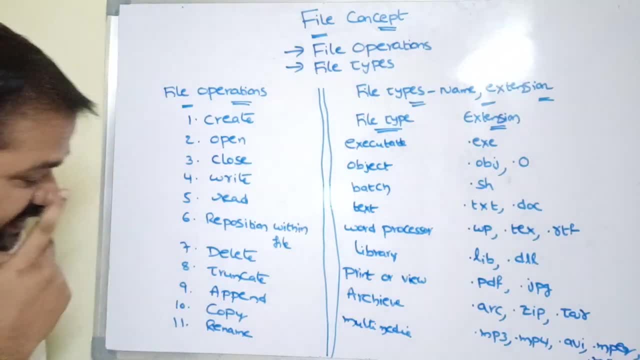 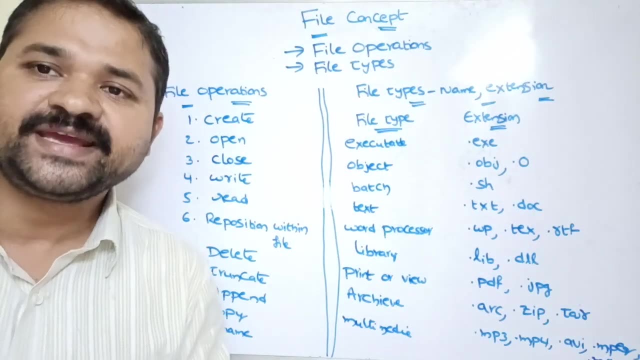 Ninth one: append. tenth one copy. eleventh one: rename. So let us see all these operations one by one. So first one is create. It is mainly useful in order to create a file. So, in order to create a file, we use create system call. 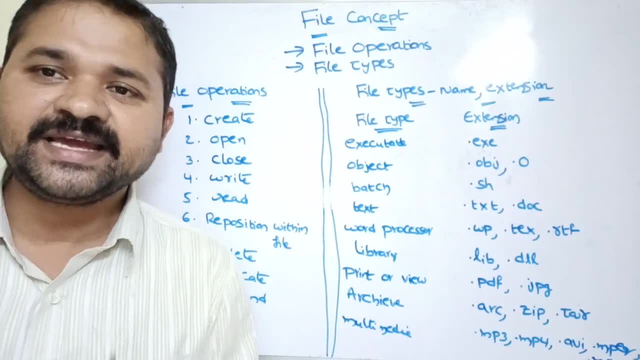 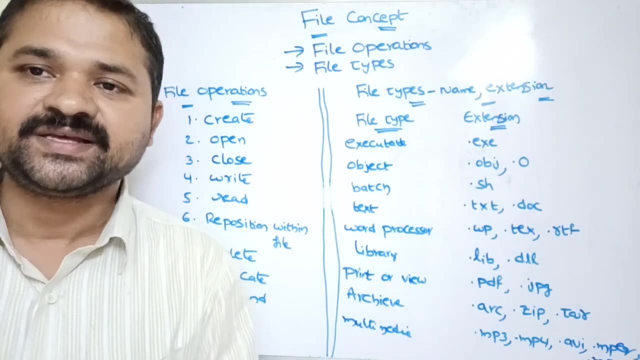 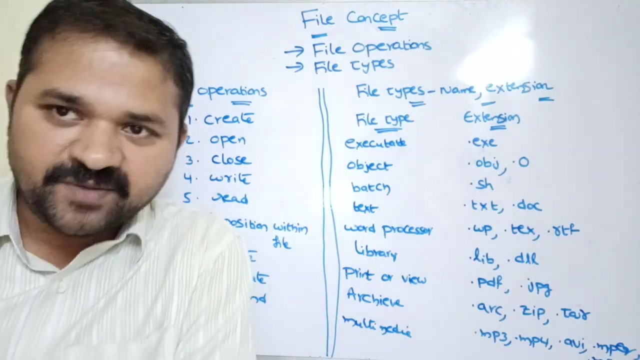 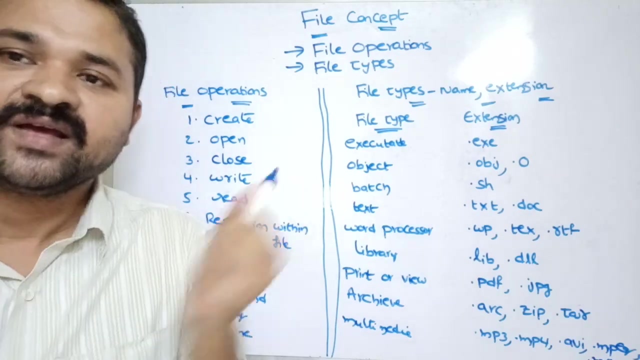 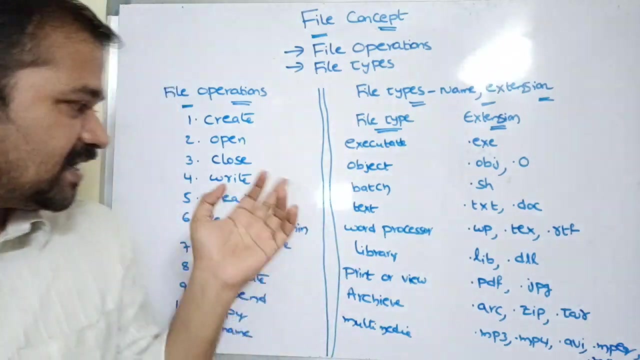 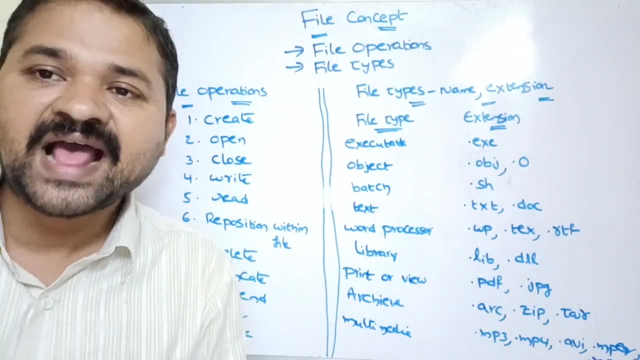 Whenever we execute a create system call, then two things will happen internally. The first one is space will be allocated for the file in the hot disk. The second one is an entry is made in the directory. So that means the file information will be stored in the hot disk along with its attributes. So those are the two steps which will happen whenever a file is created. So next one is open If you want to perform any operation on the file, like read operation, write operation, reposition operation. if you want to perform any operation on the file, first we have to open the file. In order to open the file, we use open system call. 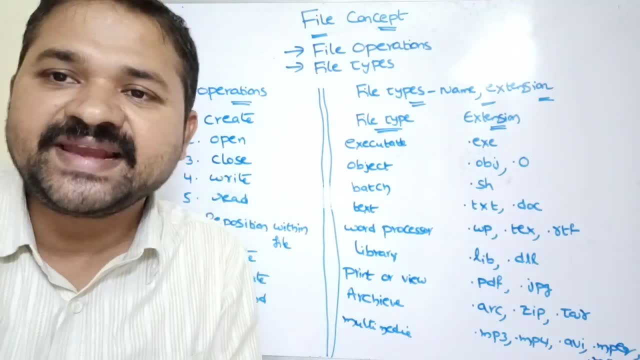 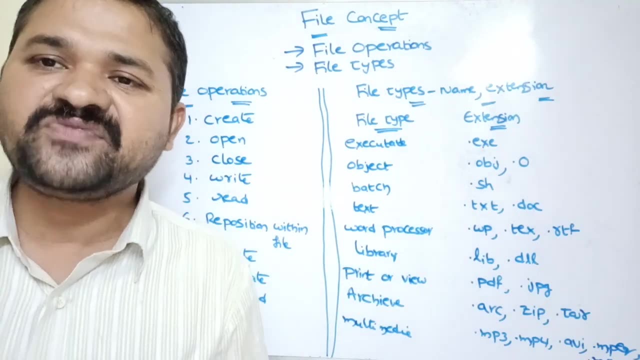 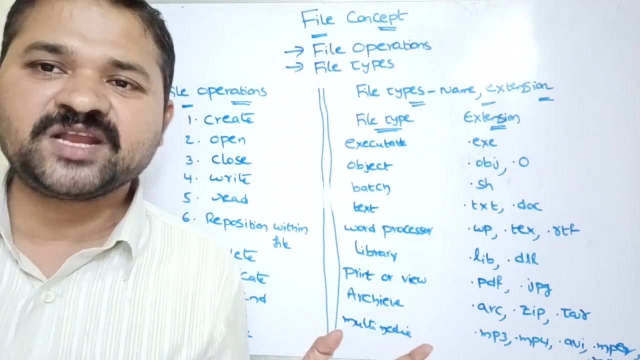 So the open system call will suggest whether the file is present in the directory or not. If the file is present in the directory, then it opens the corresponding file So that we can perform operations like read operation, rewrite operation, reposition, rename, copy, move. So likewise we can perform any operation only when the file is opened. 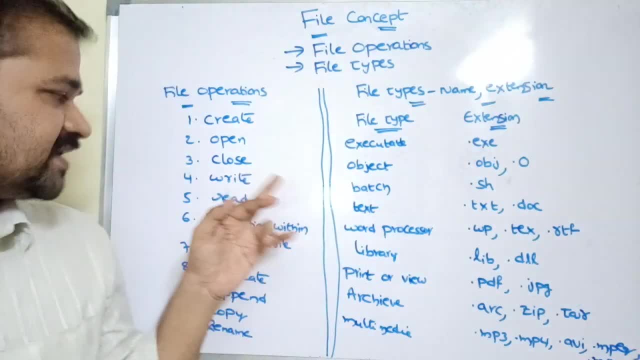 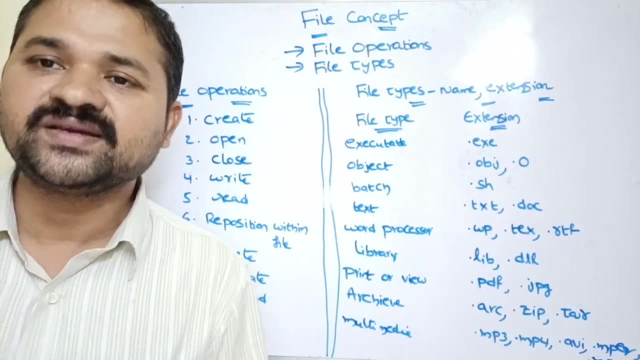 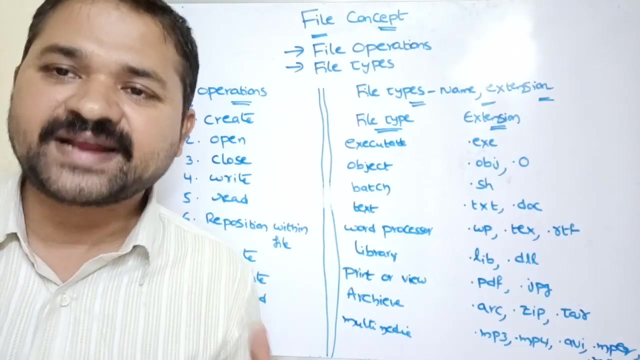 Next one is close. In order to close the file, we use close system call. the file is over, then we have to close the file. so in order to close the file, we use close system call. next one is write. before performing write operation, first we have to open the file in write. 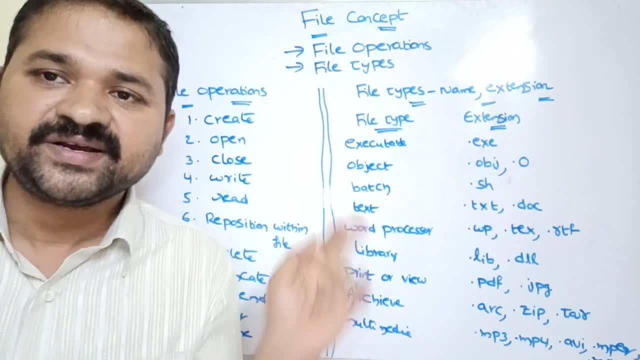 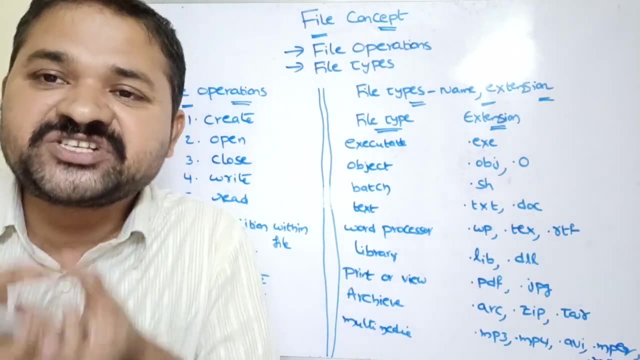 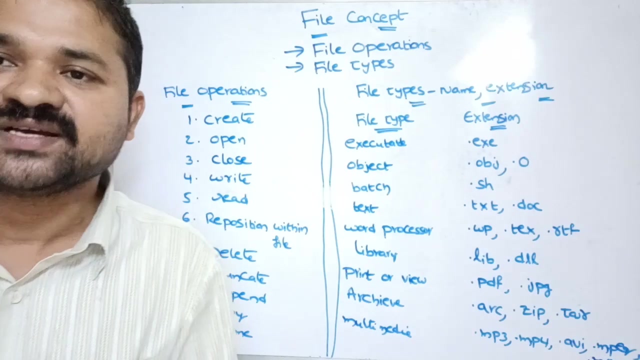 mode. in order to perform the write operation we use write system call. so here, in addition to the file name, we have to specify which data we have to write into the file. so file name as well as the data needs to be specified. so once the writing is over, then the right pointer will be moved one. 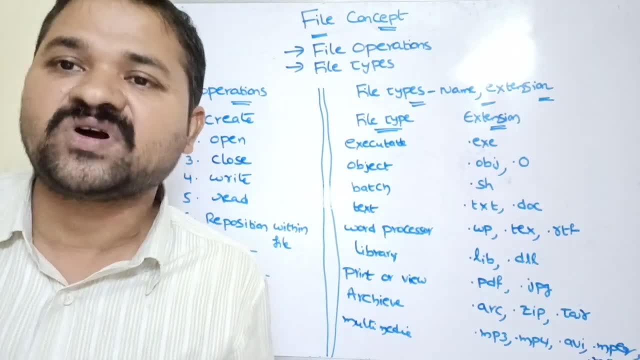 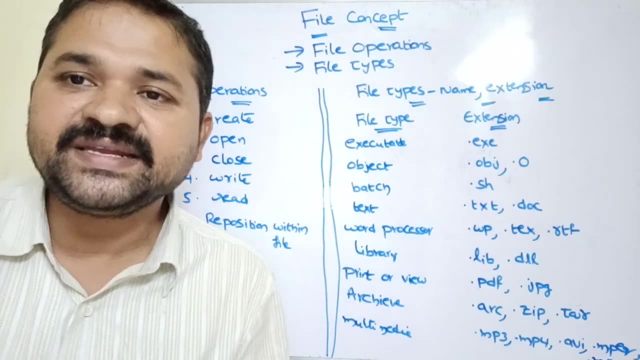 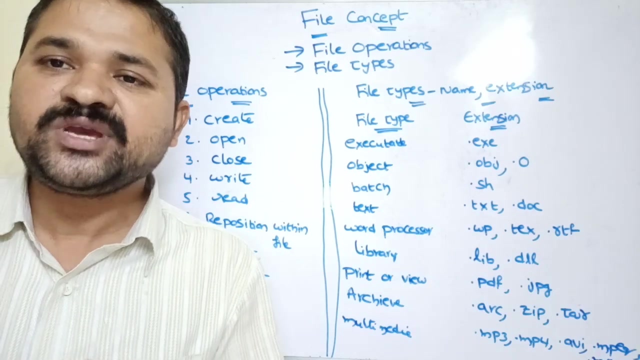 position to the right. so that means right pointer will be advanced. next one is read. so before performing read operation, first we have to open the file in read mode. next, in order to perform the read operation, we use a street system call. so here, in addition to the file name, we have to specify: 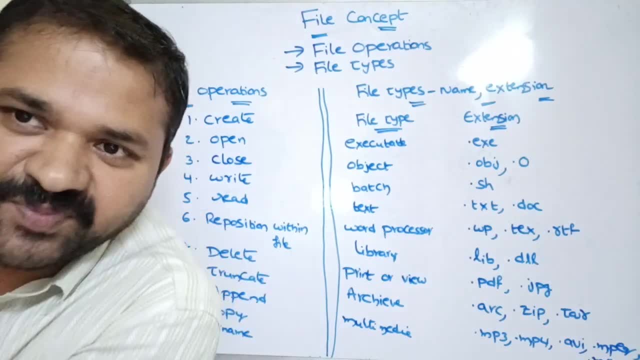 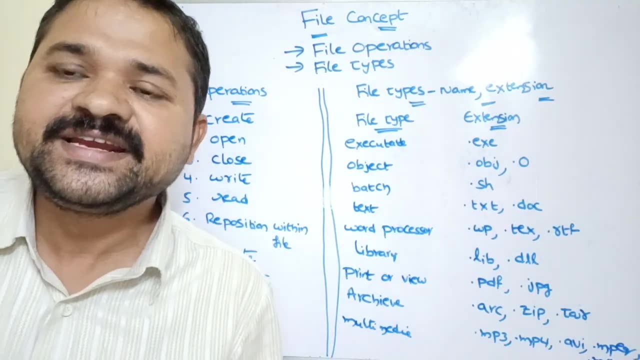 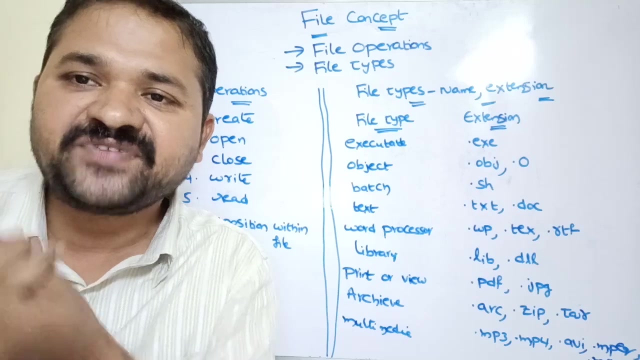 the, the variable in which the corresponding reading block will be stored. so by using read system, call or read function we can read data from the file, so that data will be stored in a variable. so in addition to the file name we have to specify that variable name also. so once the reading is over, then read. 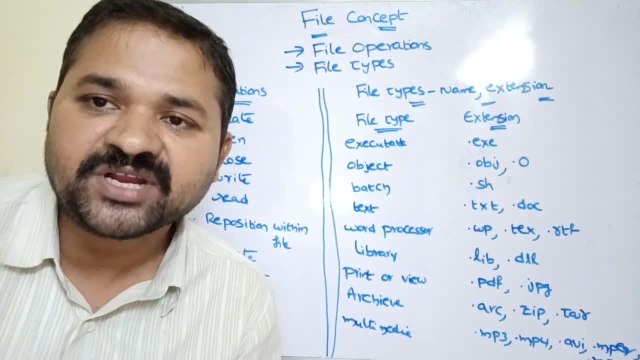 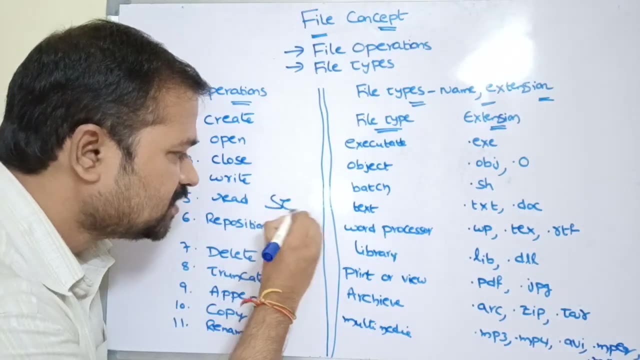 pointer will be moved one position to the right. so that means read pointer will be advanced. so next one is reposition within the file. so it is nothing but a seek function. so we know what is the use of a seek function. by using seek function we can place the 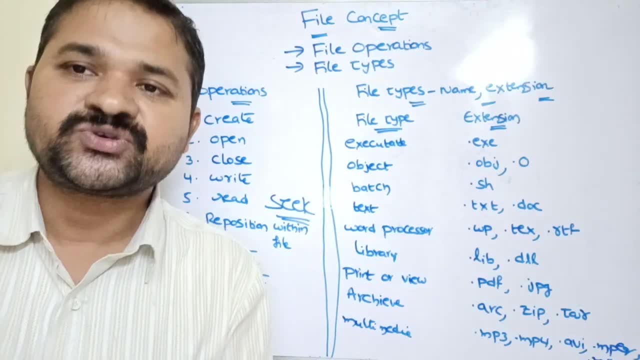 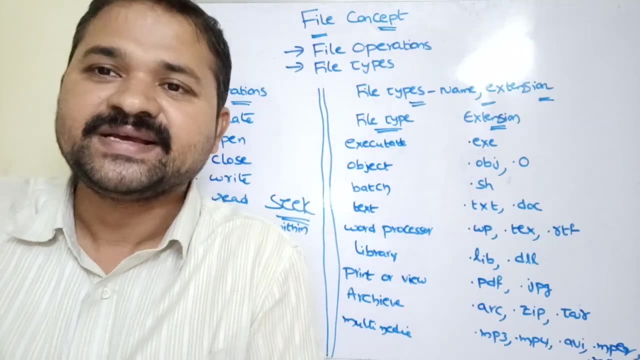 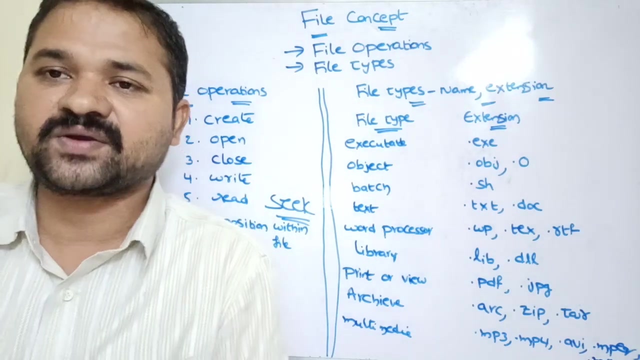 file pointer at any position as we want. so we let us assume that currently we are at 10th block and assumes that we want to move the file pointer to the 70th block, then with the help of this seek method we can move the file pointer to the 75th block here, as a reposition means it doesn't. 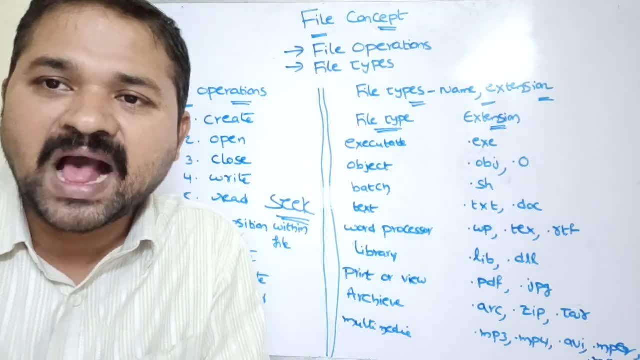 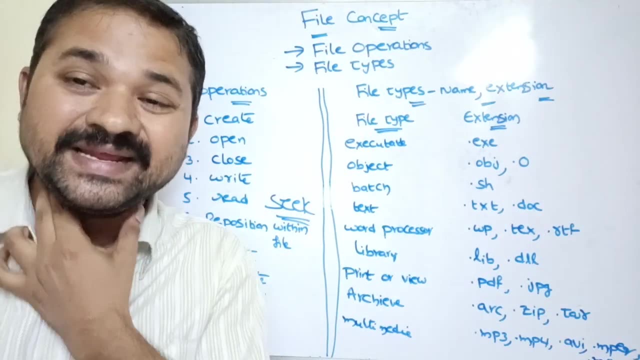 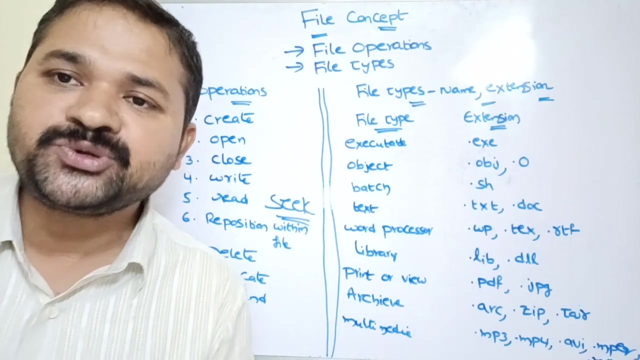 involve any read operation or write operation so we can move the file pointer to the 75th block. we have to move the pointer from one location to the another location. next one is delete. so in order to delete the file, first we have to open the file and after that, here deletion means in addition to: 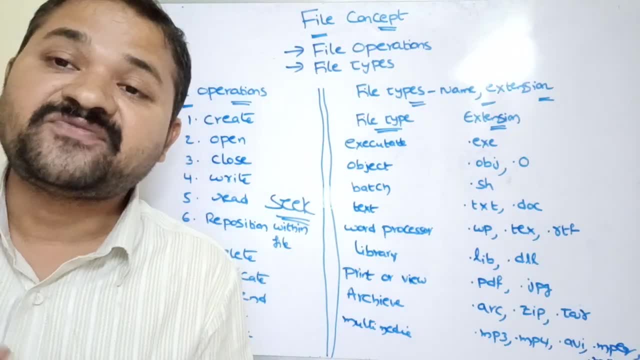 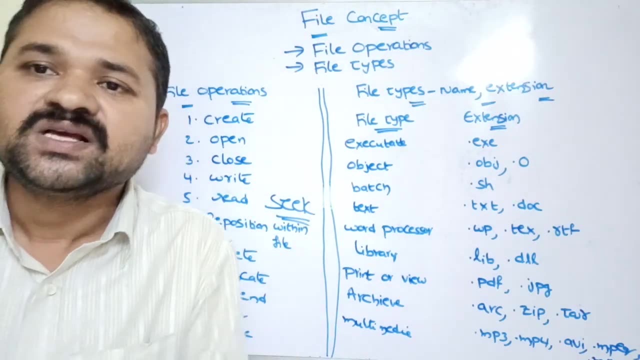 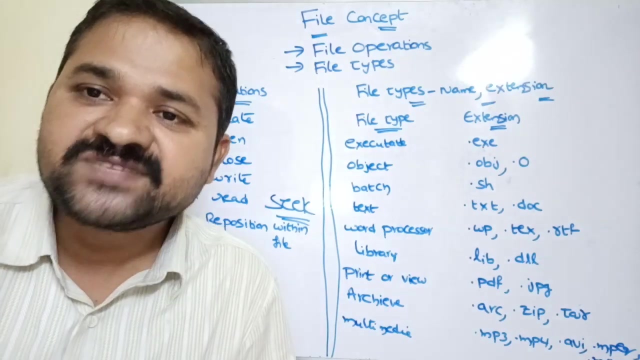 the. in addition to the content deletion, the file attributes will also be deleted, so that the corresponding allocated space will be released, so we can use that space for other file names. so here file means the contents will be deleted as well as file attributes will be deleted, so that that 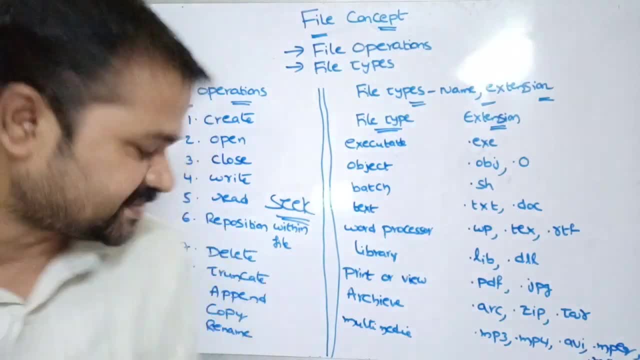 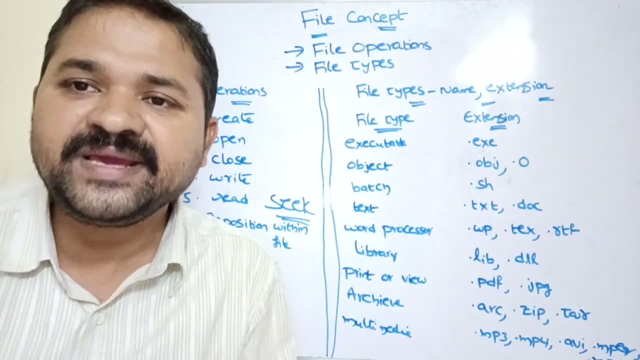 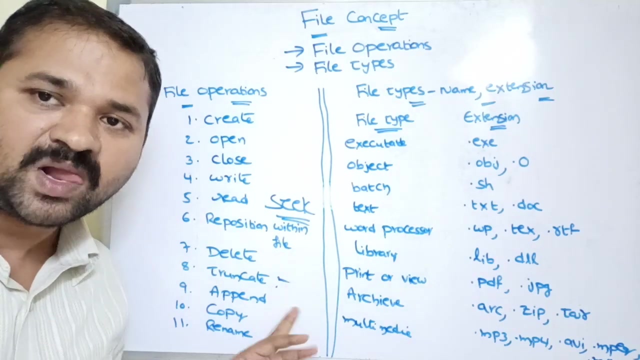 space can be used for allocating memory to some other files. next one is truncate. so truncate means only the file contents will be deleted. the file attributes will be remains the same. so so here, what will happen is the size of the file will become zero. why? because the contents of the file will be deleted and the remaining attributes are as it is. 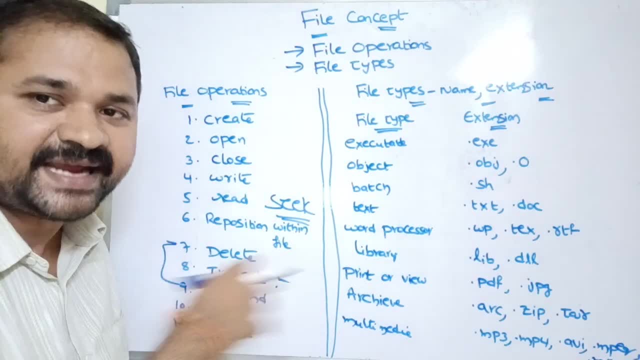 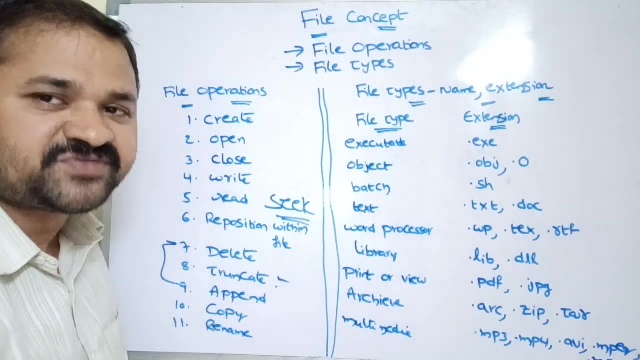 only difference between delete and truncate is: delete deletes the entire file along with attributes, whereas truncate only deletes the contents of the file. file attributes will be as it is, except size. the size of the file will become zero. next one is append. so by using append we can append some content of the file to the existing file, to the end of the file, so append. 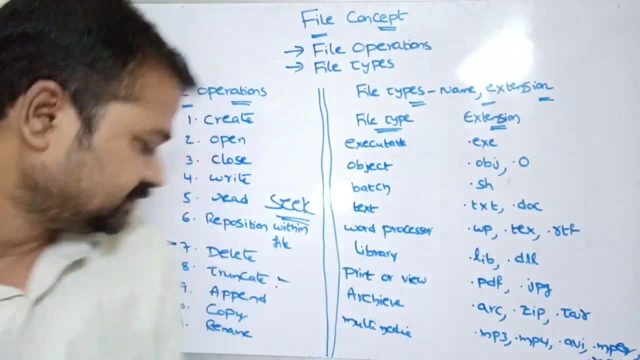 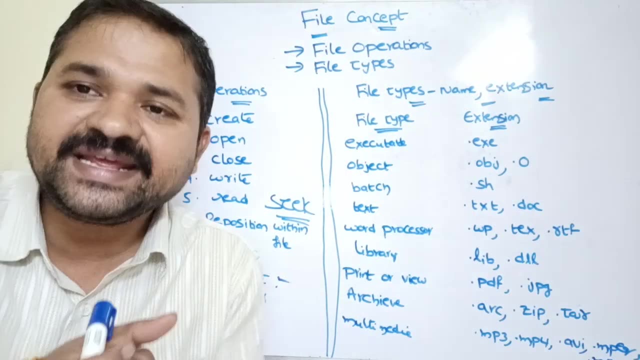 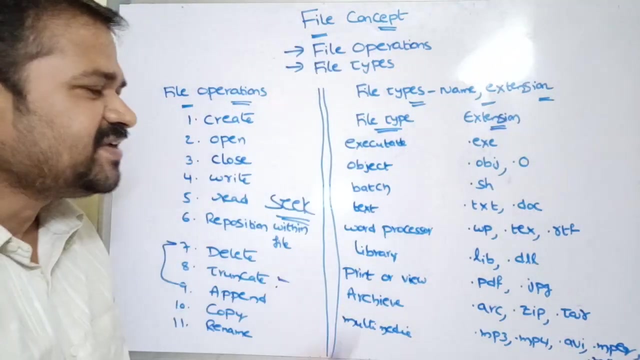 means appending some content to the end of the file. so with the help of copy operation we can copy the contents from one file to another. file rename means we can rename your file name. okay, now let's see about file types, file name with the corresponding extension. here we can have several types of files. 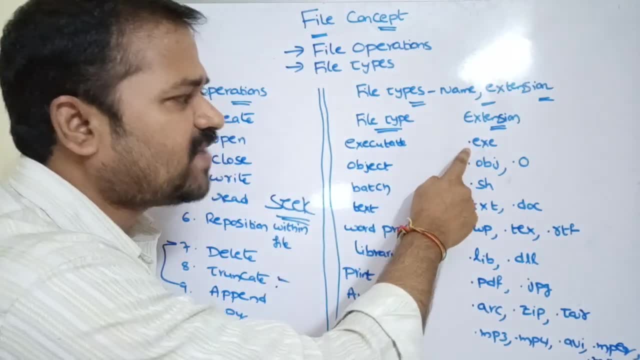 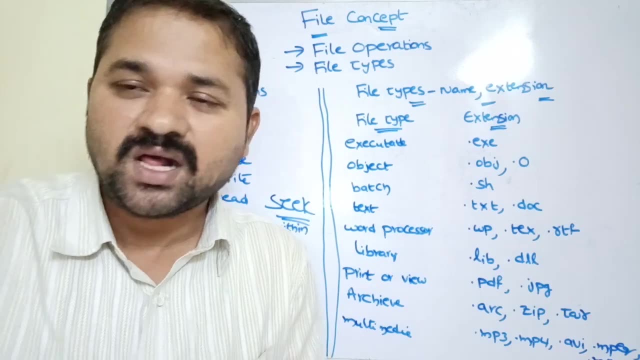 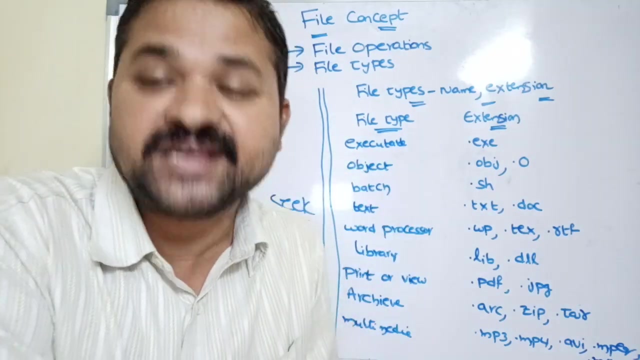 like executable file. the extension for executable file is dot exe. executable file means the corresponding file is ready for execution, so that here linker creates executable file. so whenever executable file is created, then loader loads that exam executable file into the main memory so that the corresponding program or file will be executed by 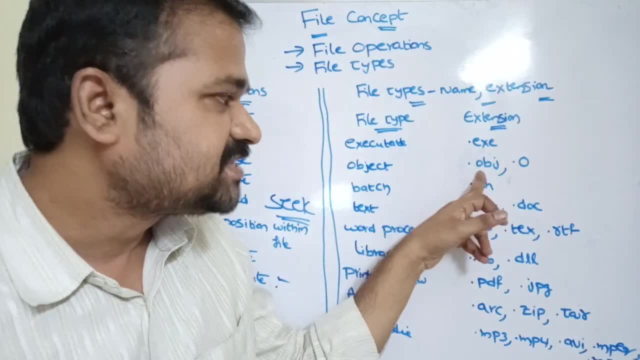 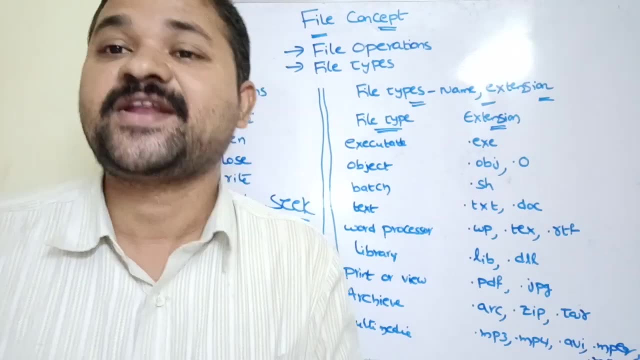 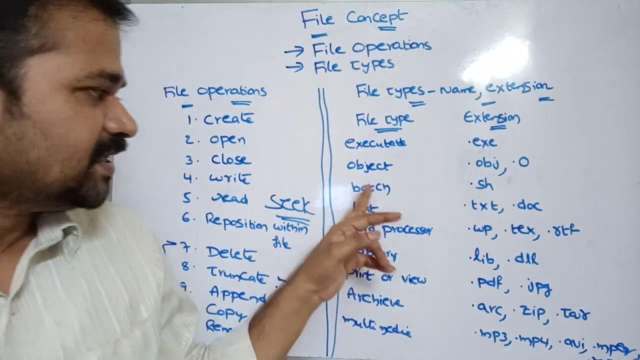 the cpu. next one is object file. the extension for the object file is dot obj or dot vo. we know what is our object file, so whenever compilation is done, then then an object file will be created. object file means it is in the terms of byte format, zeros and ones. next one is batch file. 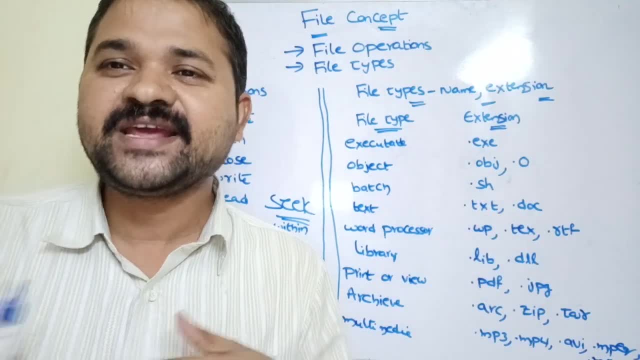 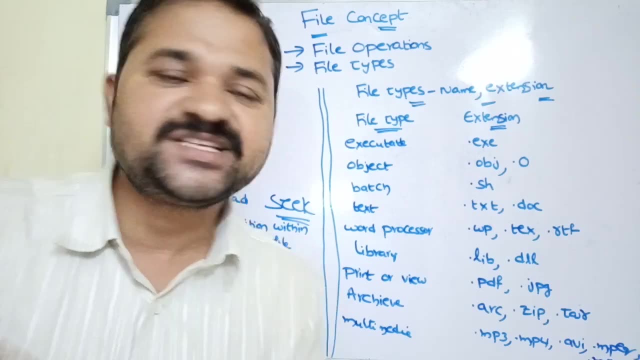 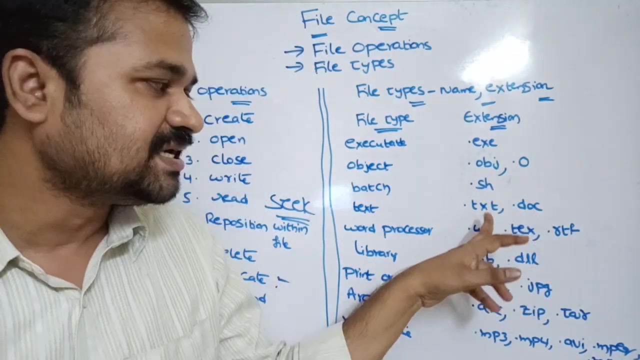 the best example for batch file is shell programming. if you take unix or linux then we will write some shell programs. so the extension for your cell programming is dot sh. next one is text file, so we can have text files like dot, exg, dot, doc. so dot text means if the 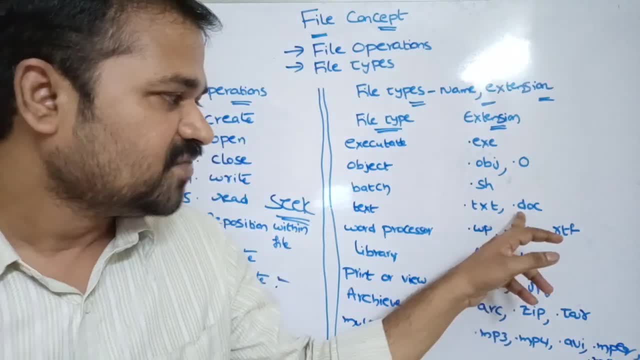 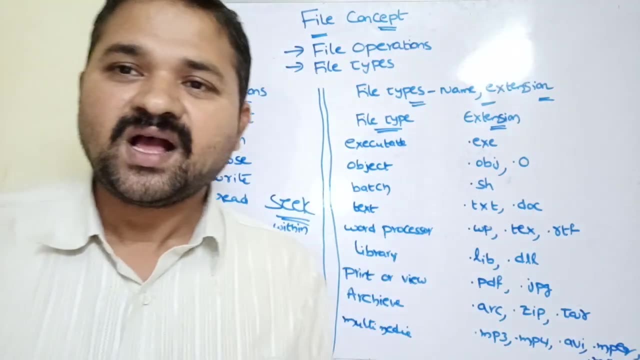 file is created with notepad, then the extension is dot txt, whereas if the file is created with microsoft word, then the extension is dot dbc. next one is word processor. we can have other types of text documents, like wp stands for word processor. we can have other types of text documents like: 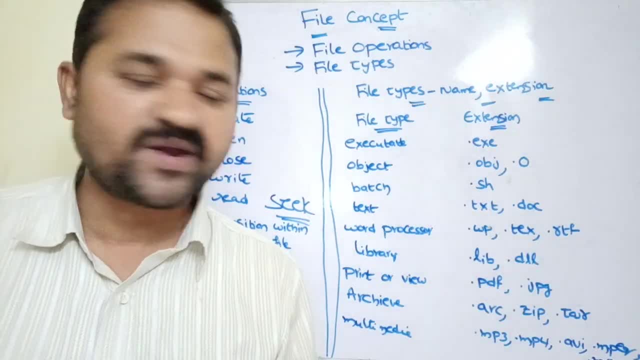 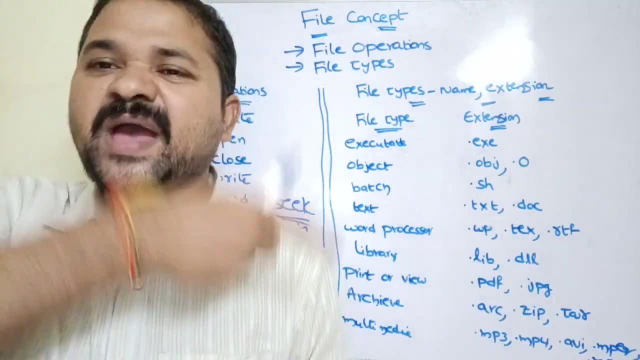 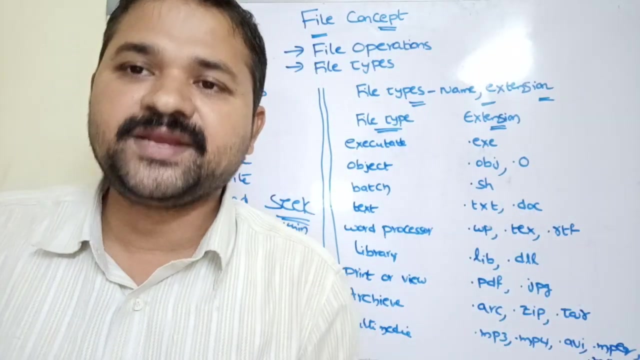 word processor: dot tx, dot ex stands for text document, dot. rtf stands for rich text format. so these are nothing but the various extensions for a microsoft word document, not only dbc. we can use these extensions also in order to: in order to give an extension for a document file, so dot. 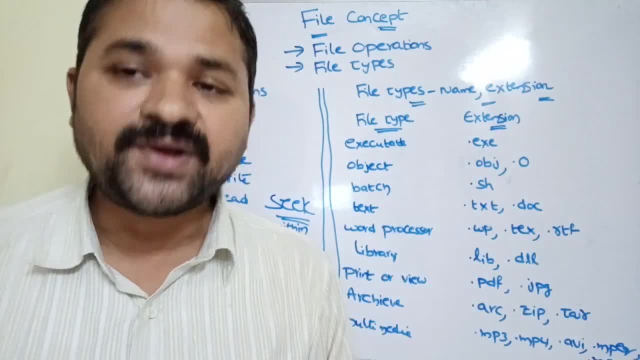 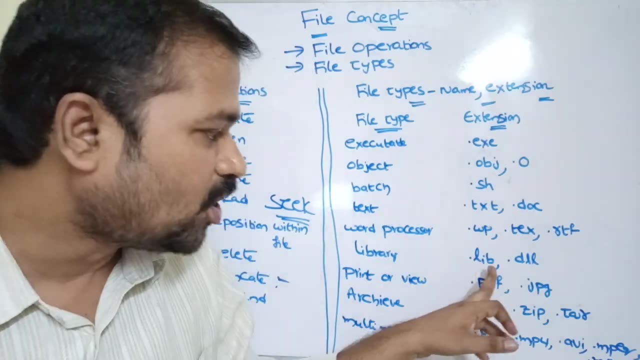 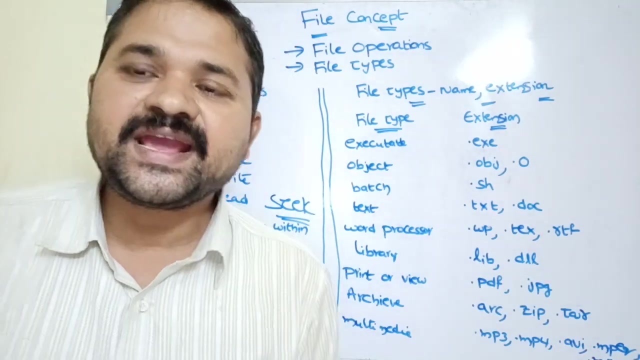 wp word processor, dot, ex text format, dot, rtf, rich text format. and next one is library file. now we can have several library files like dot, lib, dot, dynamic linking library, so these library files are mainly useful while linking. if you take ash, include math dot h, it contains several mathematical 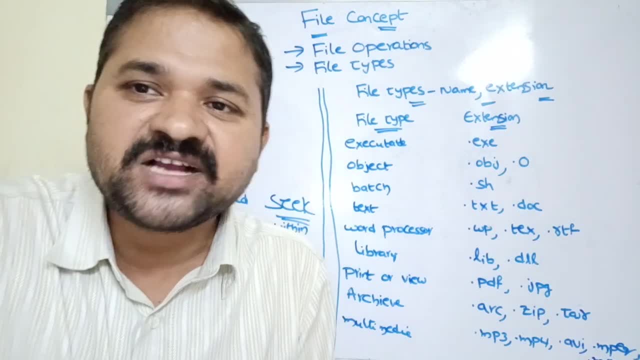 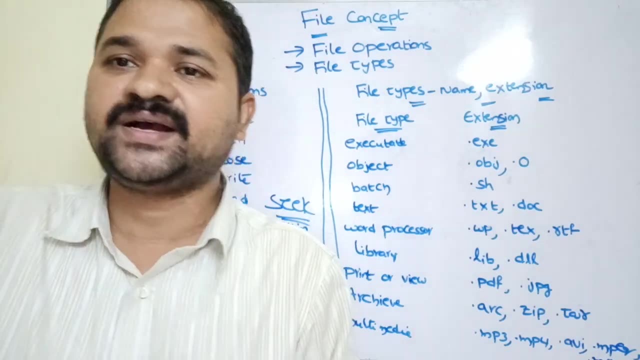 functions like sine x, cos x, but actually every function has a library file, okay, so whenever we want to execute that function, then that library file will be executed during execution. so that is the need of library file. the extension for your library file is dot, lib or dot. 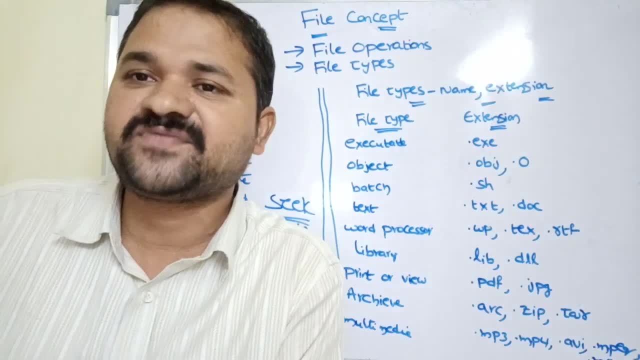 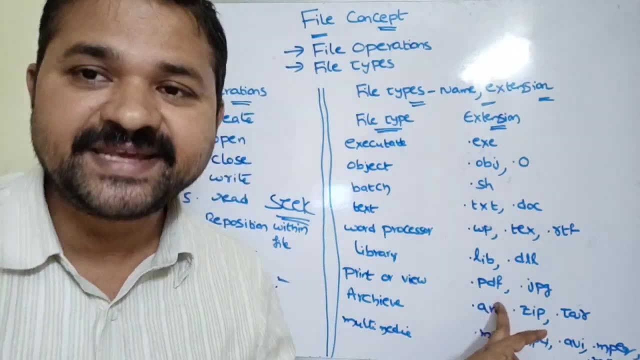 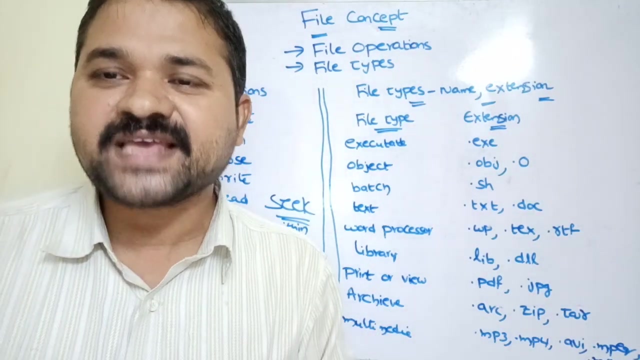 dll, so every library function contains a library file. next one is printer view, so in order to view the contents of the file, we use this dot pdf or dot jpg files. next one is archu, so so we know what is archu. it contains a collection of related type information. we can have several types of 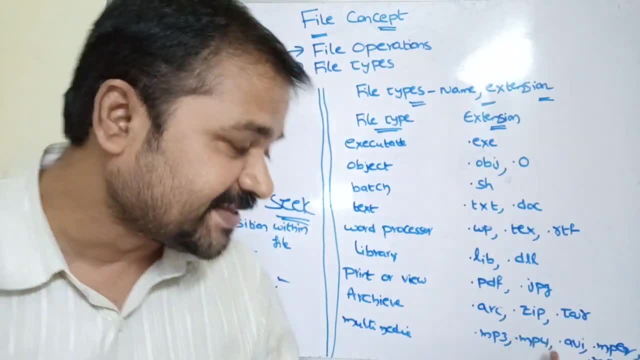 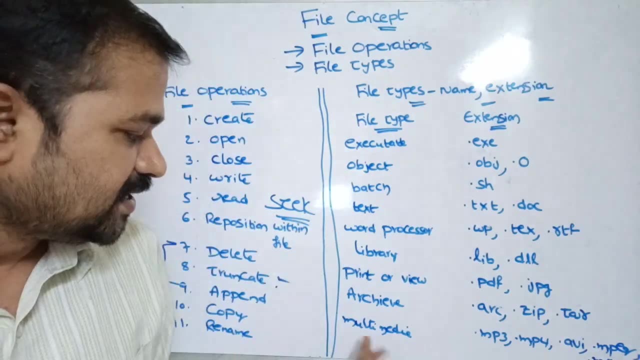 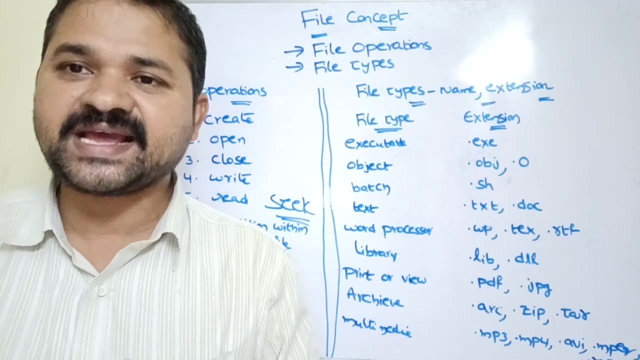 actual extensions like dot arc, dot zip. next one is dot tape, archu. so these are the various extensions in order to create an archu file. next one is multimedia, so here multimedia stands for only video files. here we can have several types of extensions like dot mp3, dot mp4, dot avi, dot mpeg. 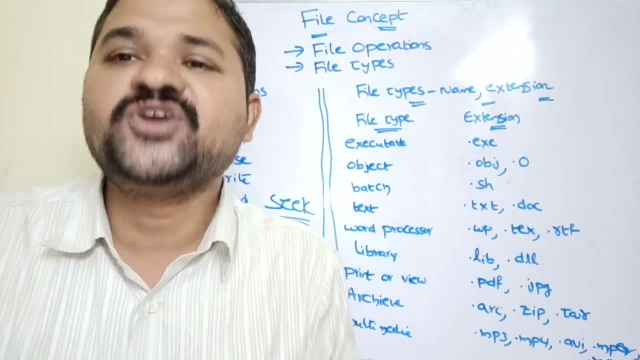 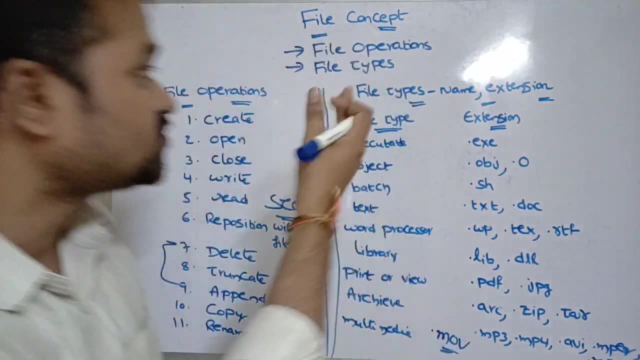 if you take iphone, if you create a video with iphone, then the extension is dot mbov, dot mbov. so these are the various extensions of a file and the various operations that we can perform on the files. so